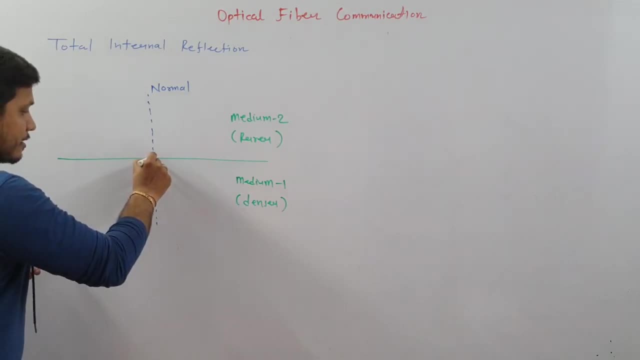 and now here. if ray enters from here, right, and what will happen is like, if ray is entering like this and if i say this is what angle of incident i, then when ray enters from denser medium to rarer medium angle of refraction, that will increase. so we'll be finding this is what the 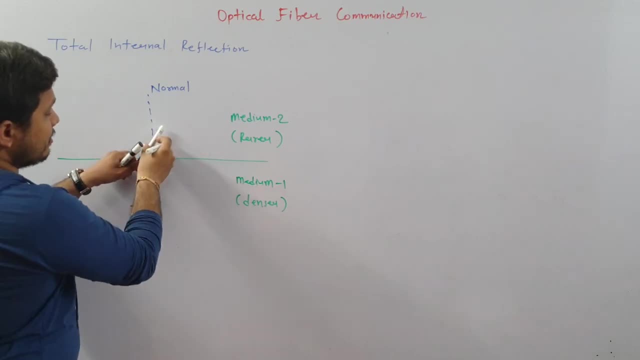 basic trajectory, but here this angle will increase with respect to angle of incident. so you'll be finding it will go like this: now: if i further increase this angle of incident, you'll be finding this ray that is bending away from the normal right now at one angle. 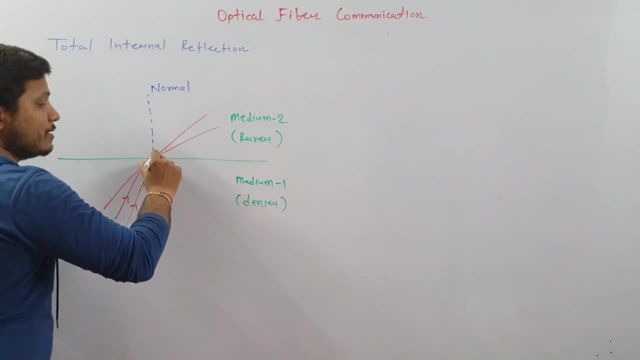 what will happen is like: this angle will be parallel to the surface. so that angle which is parallel to the surface after having refraction, that angle is critical angle. so at critical angle you'll be finding this angle of refraction that is 90 degree. so here, at critical angle, 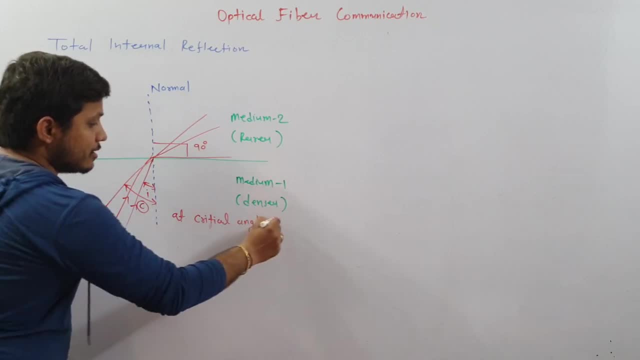 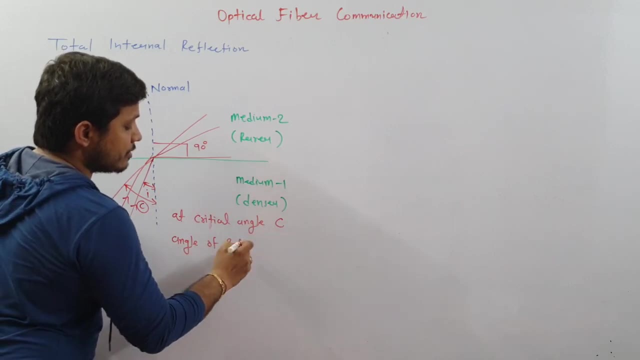 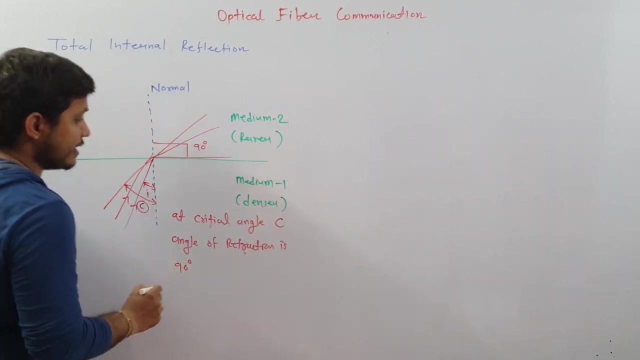 then you have angle of refraction. in this particular episode your angle of refraction is 90 degree. so when the ray enters from denser medium to rarer medium, angle of refraction will be greater than angle of电. So when ray enters from denser medium to rarer medium, angle of refraction will be greater than angle of電. 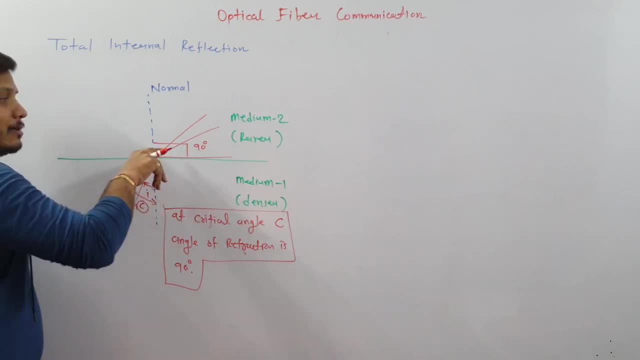 of incident but at critical angle, that angle of refraction that will get to 90 degree. that's why that angle of incident that is called as critical angle. now see why it is called as an critical angle. so to understand that if I have angle grid angle of incident greater than critical angle, so if angle of incident that is 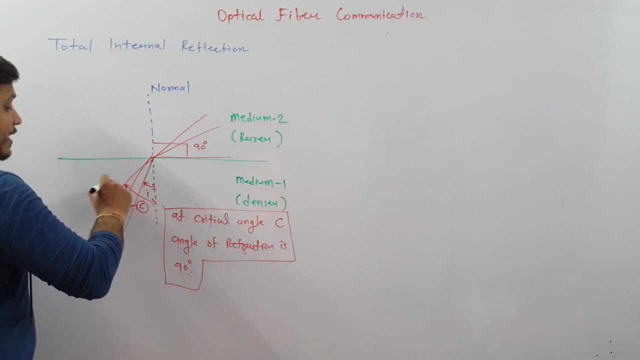 greater than critical angle. so in that case you will be finding that ray is getting reflected back. so if angle is greater than critical angle, that ray will get reflected back into the medium. so that's why this angle of incident at 90 degree of angle of refraction is called as critical angle. so that should. 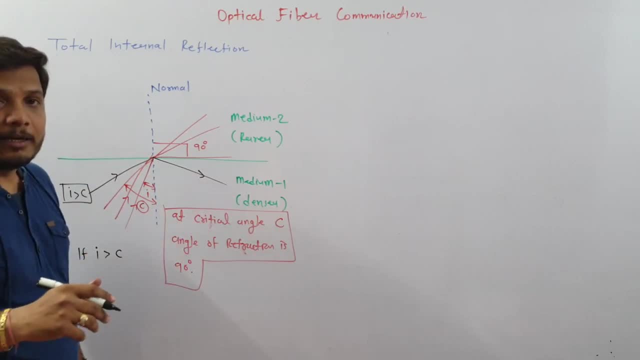 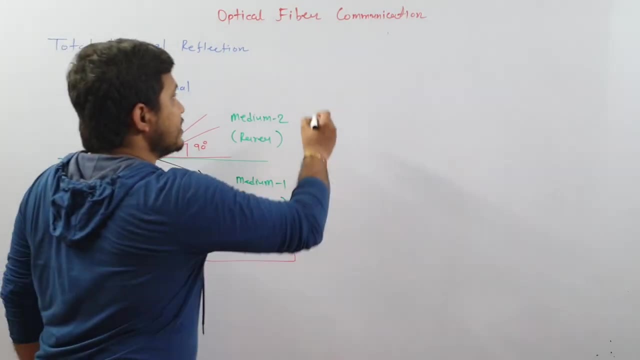 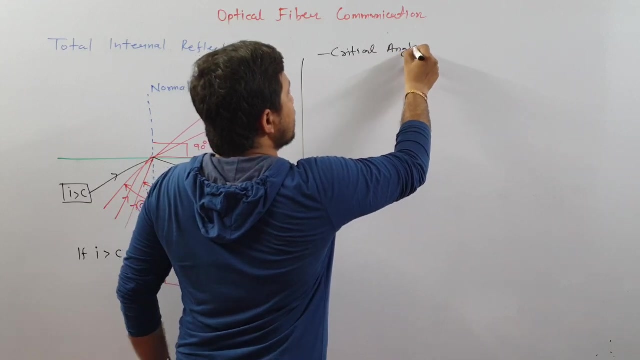 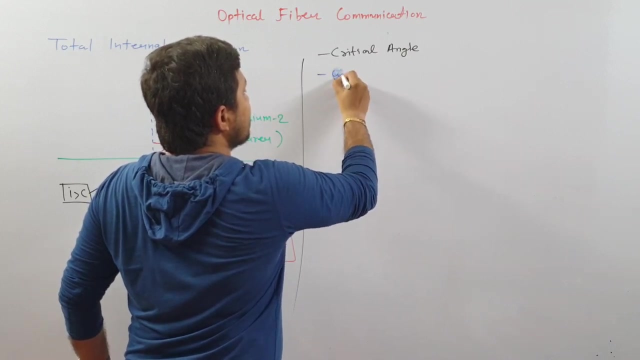 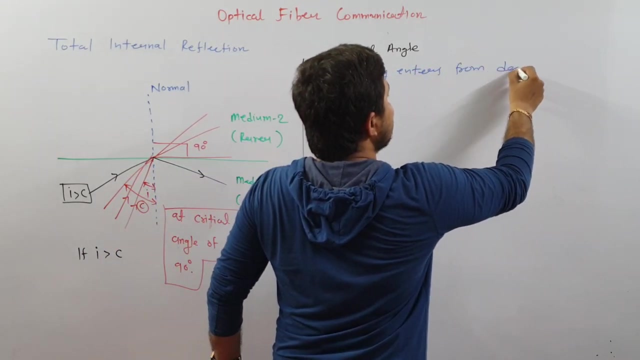 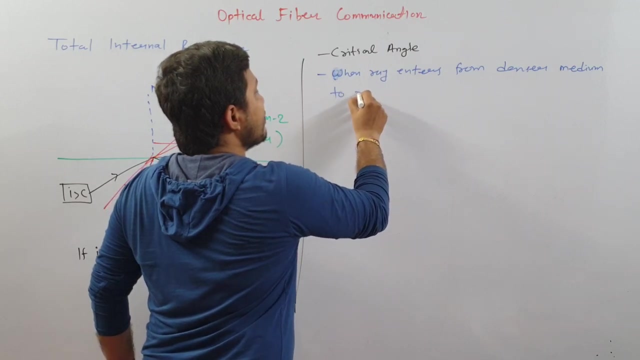 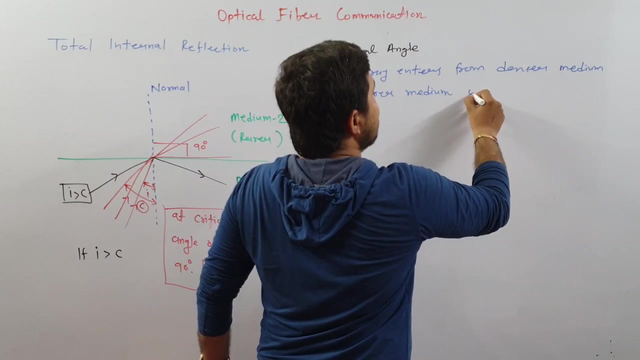 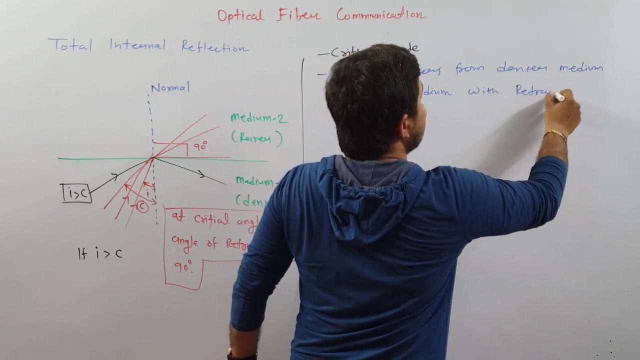 be clear to all what is critical angle. critical angle is angle where angle of refraction is getting 90 degree. so let me write the definition. what is critical angle? so critical angle? it is a angle when ray enters from from denser medium to rarer medium with refracted angle of 90 degree. 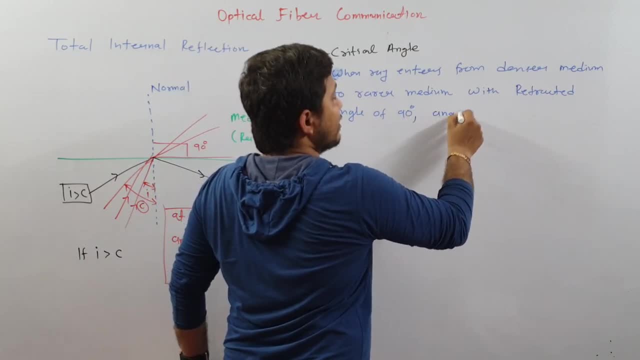 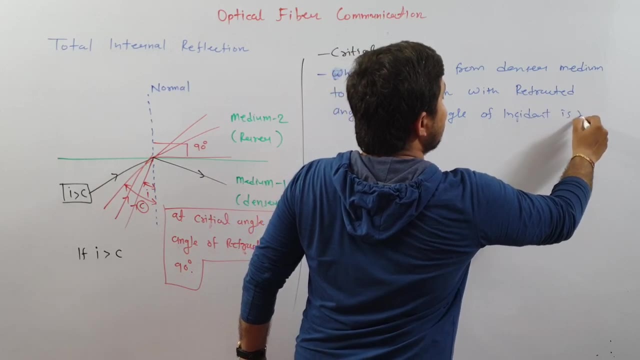 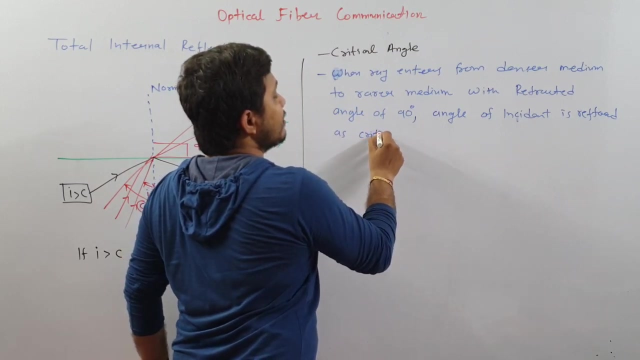 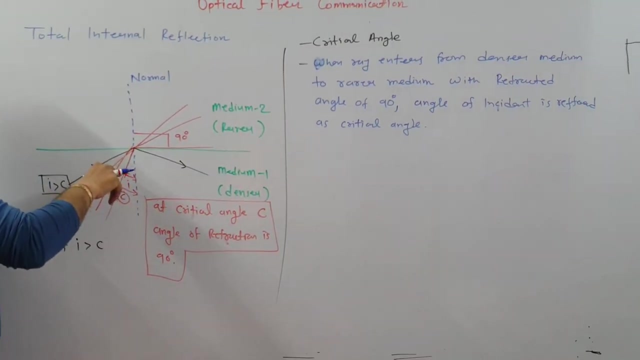 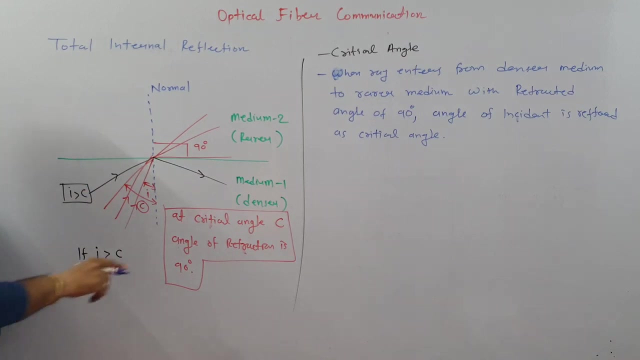 So angle of incident is referred as critical angle. So when you have angle of incident such that angle of refraction is 90 degree- that is, when you have angle of refraction is 90 degree- that angle of incident is referred as critical angle. 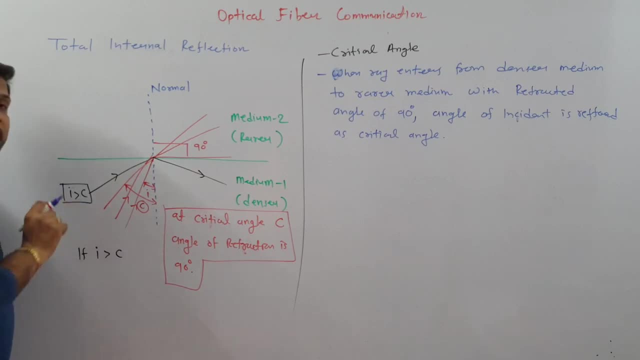 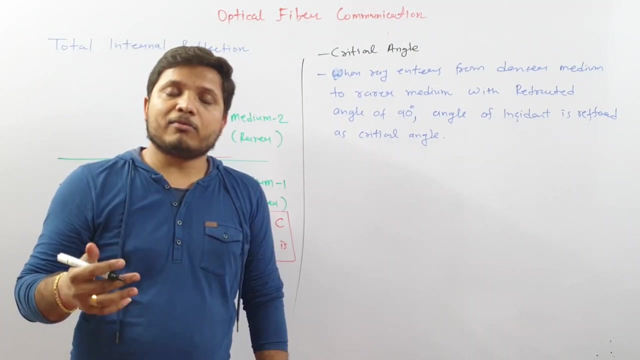 And if you increase angle of incident greater than critical angle, there will be total internal reflection. Now see why this is total internal reflection. What is total internal reflection? So, first of all, in reflection, what happens is like you have surface which is reflective surface. 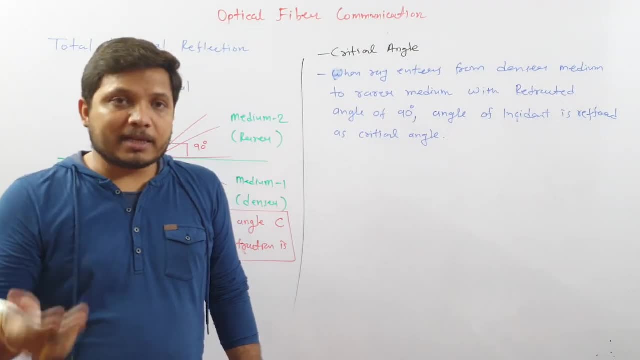 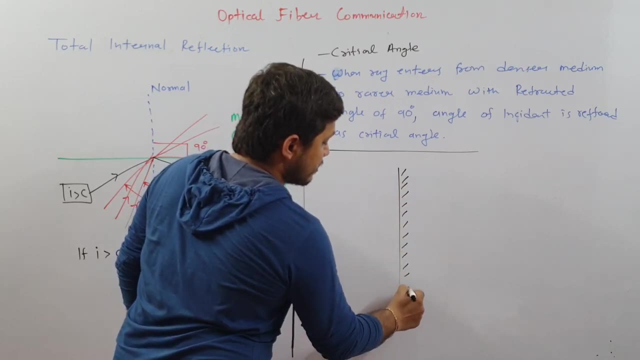 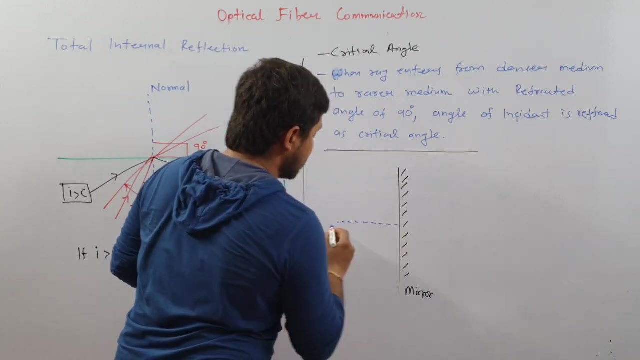 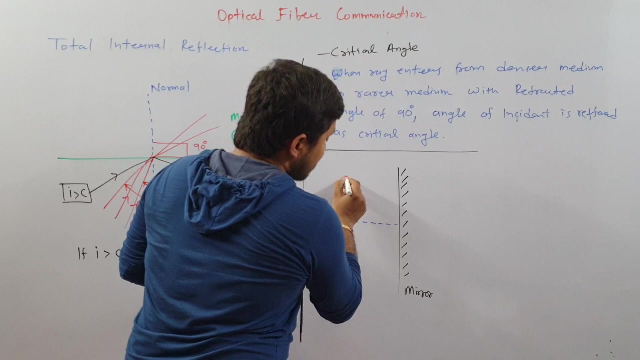 One can say it is mirror. So in mirror in case of mirror, if I say this is mirror And if I say this is marble, So in case of mirror, what happens is when this light is reflecting from this mirror. 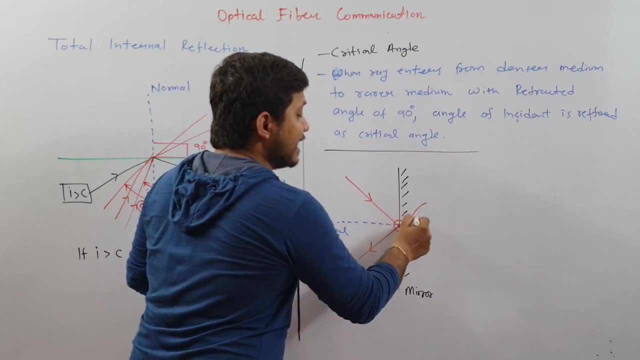 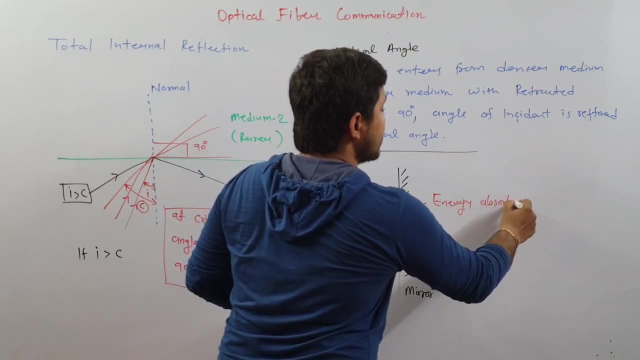 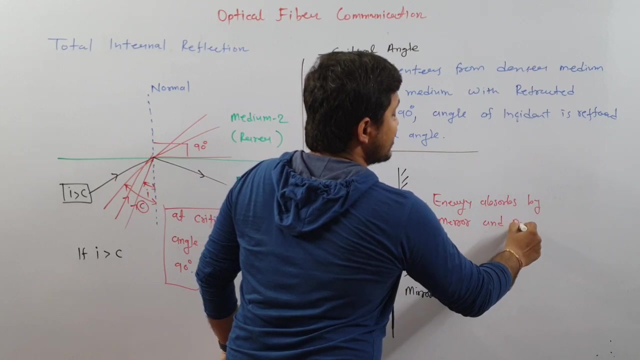 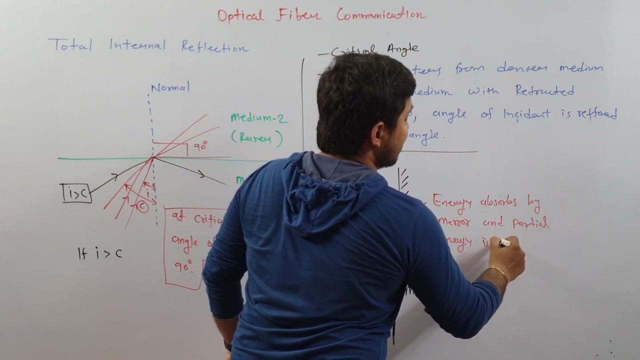 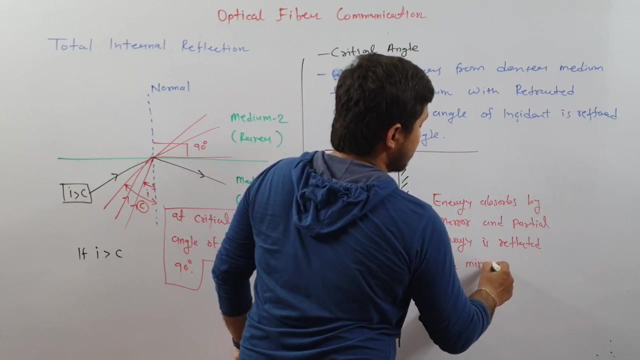 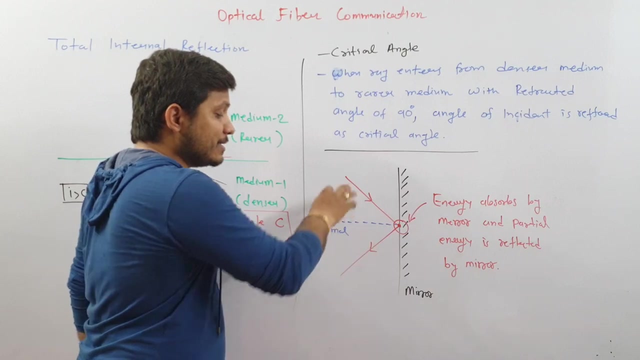 there will be somewhat energy that is getting absorbed by mirror, Energy absorbed by mirror and partial energy is reflected by mirror. So in case of mirror, some what energy is getting absorbed here on the surface when signal ray is getting reflected, While in case of total internal reflection? 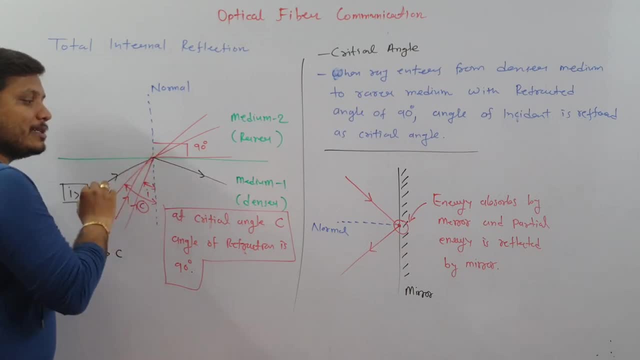 there will be no absorption of energy, Total energy that will get back into the medium from where we are inserting the signal. So here, total signal energy that is getting reflected back, as if you provide angle of incident which is greater than critical angle. 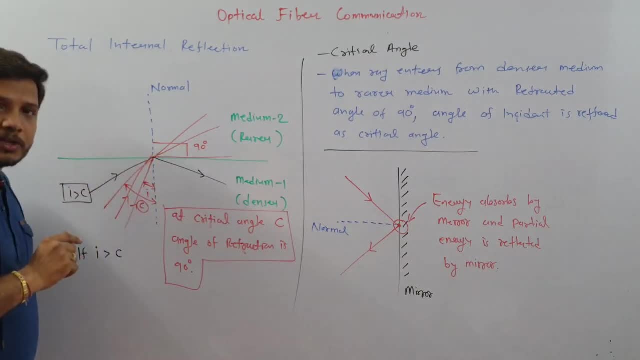 That's why this is what total internal reflection, Why it is internal. The reason is it: ray is traveling in the same medium, Right? So ray is traveling in the same medium and there is a reflection. and that is what total reflection. That's why it is total internal reflection. 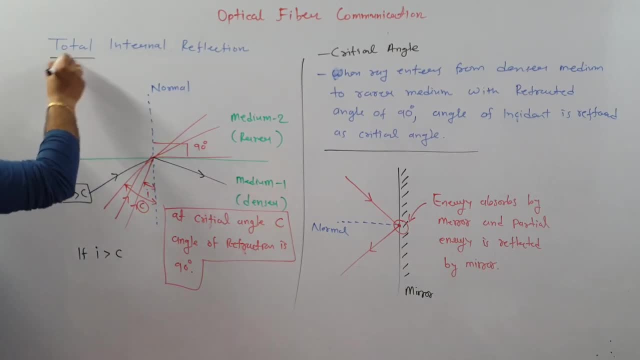 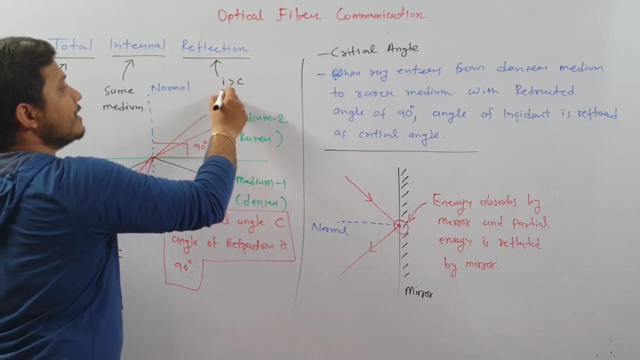 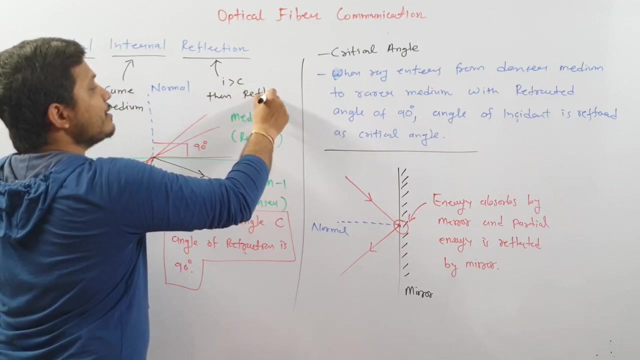 See why total Total? because of total energy, Why it is internal. It happens in the same medium and if angle is greater than critical angle, if angle of incident that is greater than critical angle, then there will be reflection. So this is what total internal reflection. 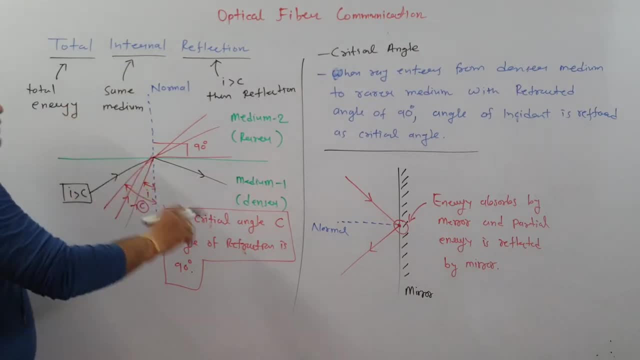 So this is what total internal reflection. So this is what total internal reflection. Here there is no absorption of energy on the surface. Here there is no absorption of energy on the surface. So this should be the clear to all like See, in case of total internal reflection. 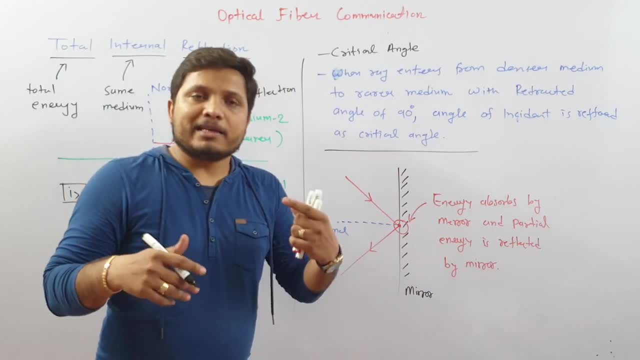 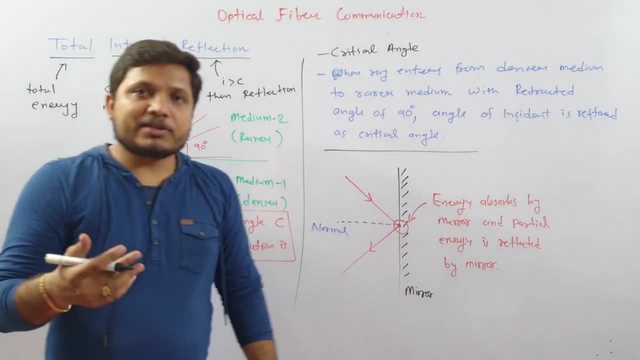 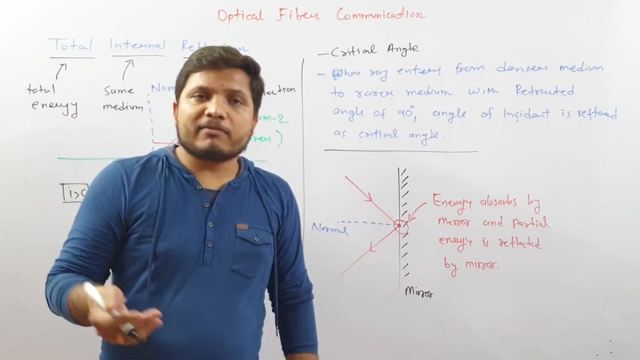 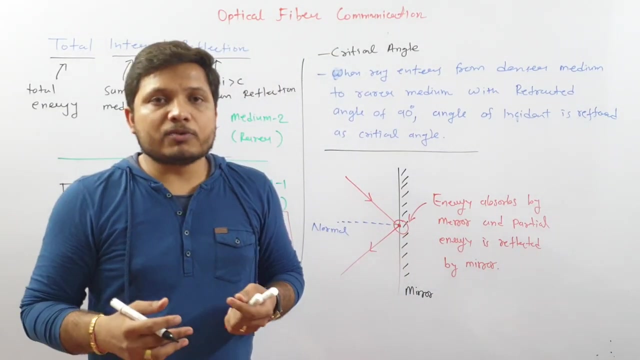 There is no absorption of energy, while in case of reflection by mirror, You will be finding there are so many applications and those applications are used in so many practical real life applications Like optical fiber communication. so that is what the subject where we use total internal reflection in prism, we use total 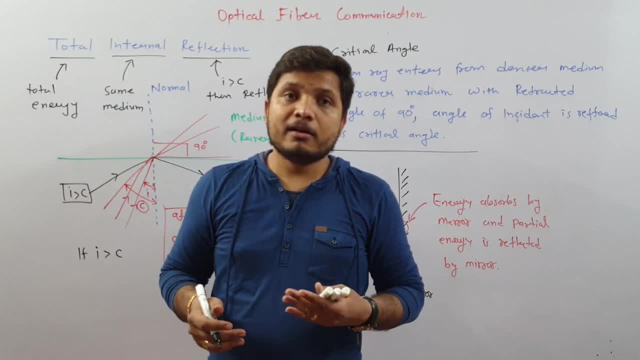 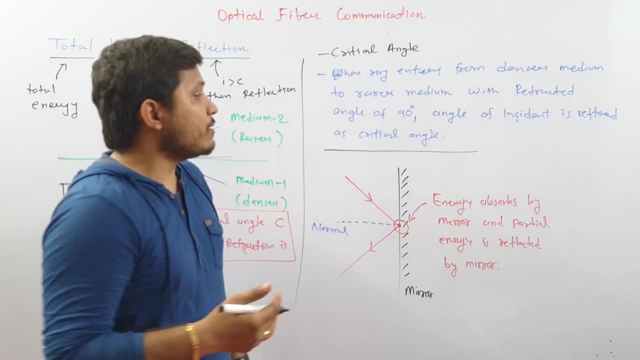 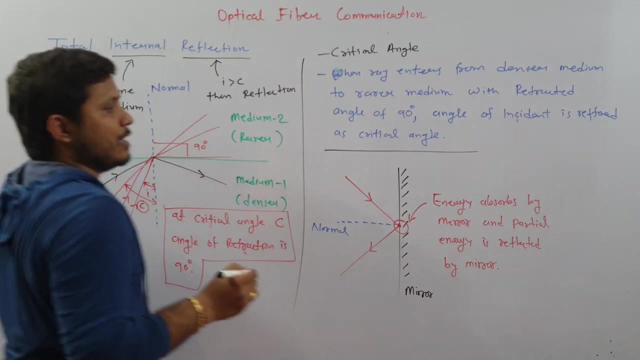 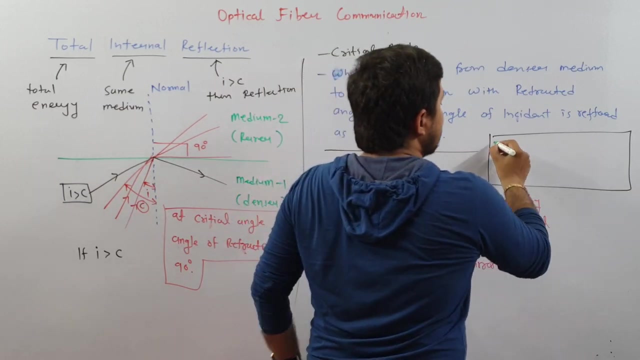 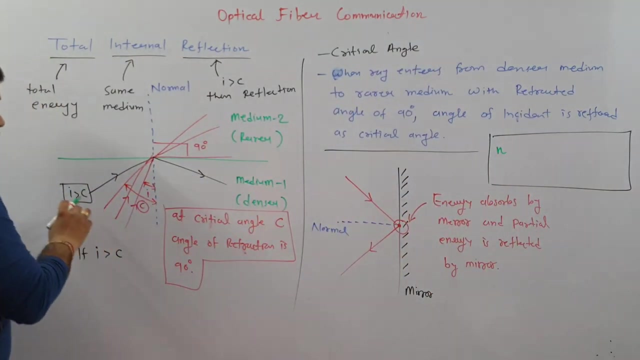 internal reflection, you'll be finding glittering of diamond. so that is what explains you how total internal reflection is happening. and now somewhat mathematics that we should know. based on this total internal reflection as per snail slope, as per snail slope, as per snail slope, we can say refractive index. see here: signal enters from denser medium right. 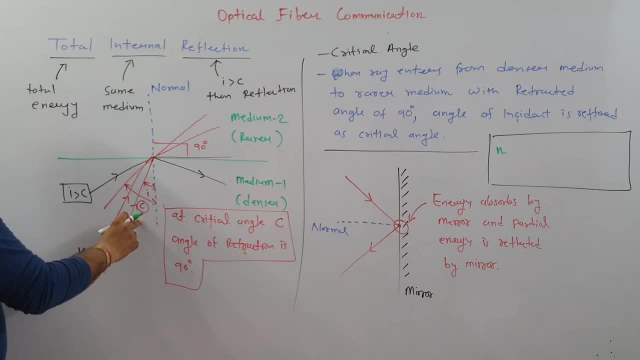 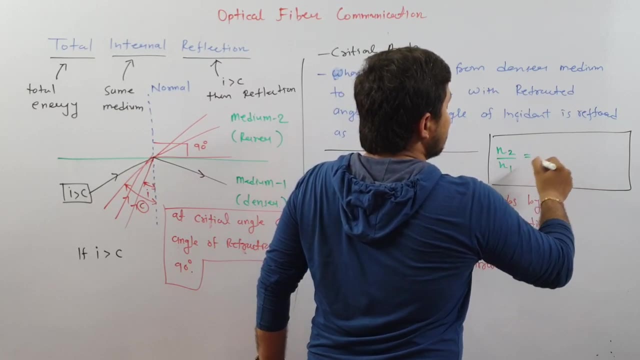 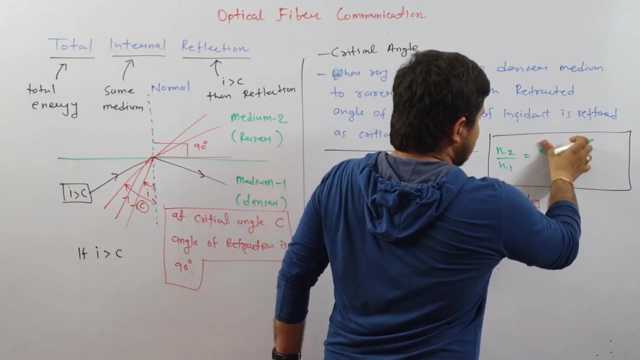 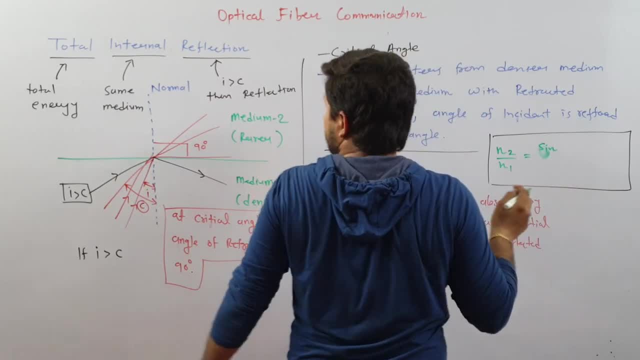 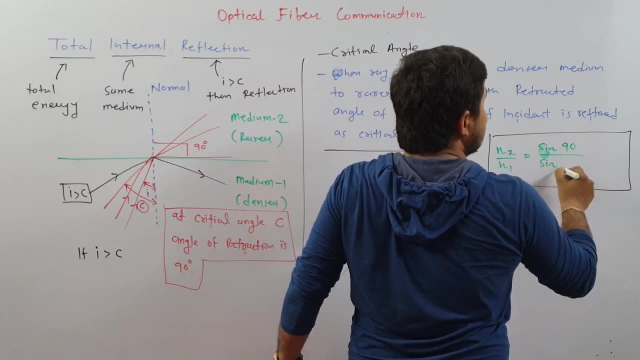 sine of that medium 2 angle, that is 90 degree. sine of that medium 2 angle, that is 90 degree. sine of that medium 2 angle, that is 90 degree. and and and sine of this angle, that is critical angle. sine of this angle, that is critical angle. 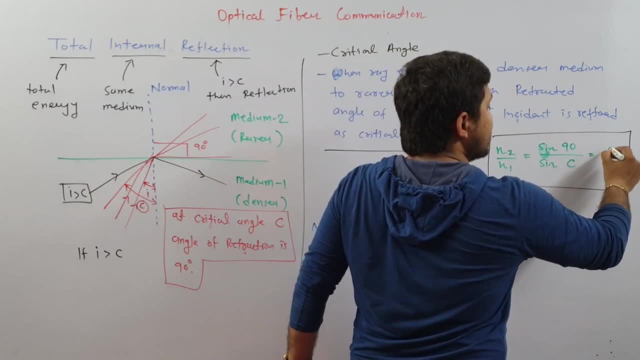 sine of this angle, that is critical angle, right. so this sine 90, that is one. so this right. so this sine 90, that is one. so this right. so this sine 90, that is one. so this will be 1 divided by will be 1 divided by. 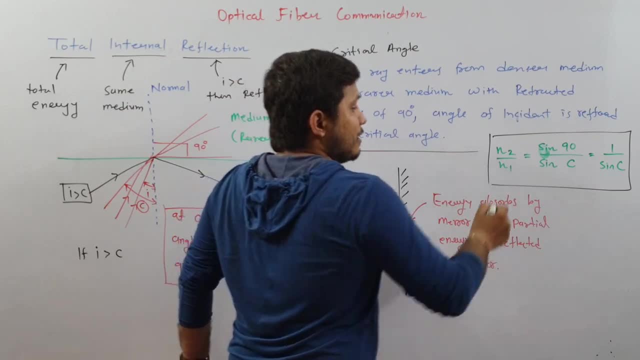 will be: 1 divided by sine c, so n2 by n1. sine c, so n2 by n1. sine c, so n2 by n1. n2 by n1, that is what relative refractive. n2 by n1, that is what relative refractive. 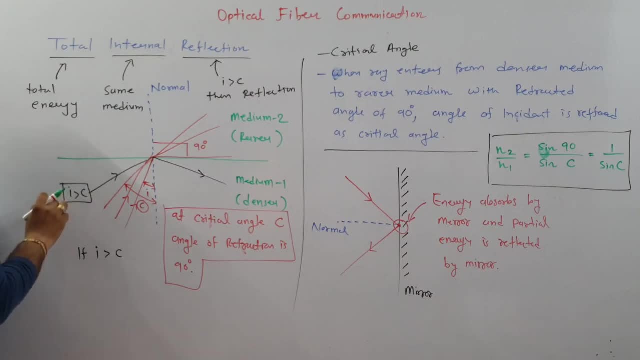 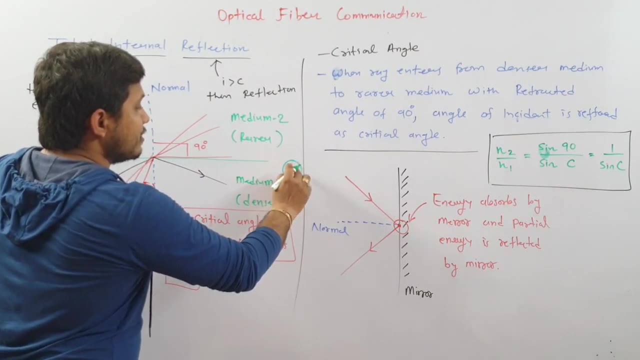 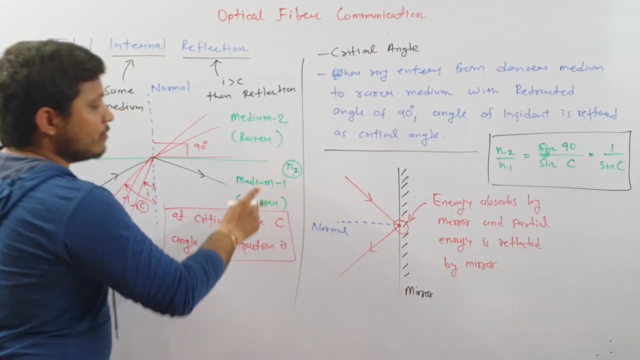 n2 by n1. that is what relative refractive index index of medium 1, right? so sorry, i have mistaken. if i say this is what refractive index n1- sorry n2- for this medium 1, then this is correct. so i am considering medium 1's refractive index is 2. 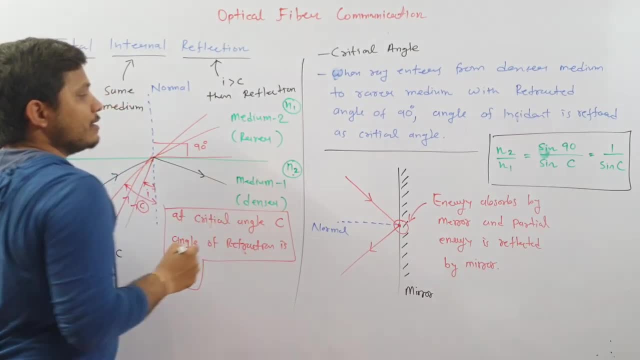 and medium 2's refractive index is 1. right, in that case one can say: n2 by n1 means refractive index of medium 1 divided by refractive index of medium 2, that is, sine 90 by sine c, as per snail's.